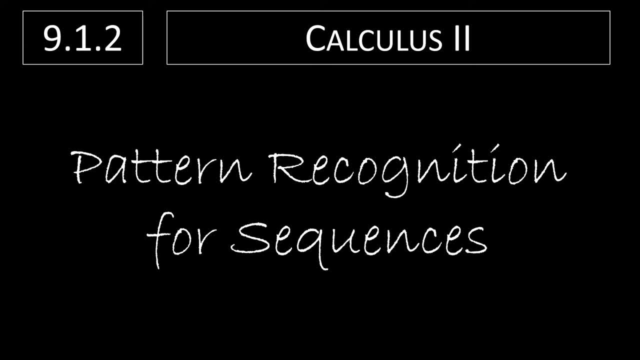 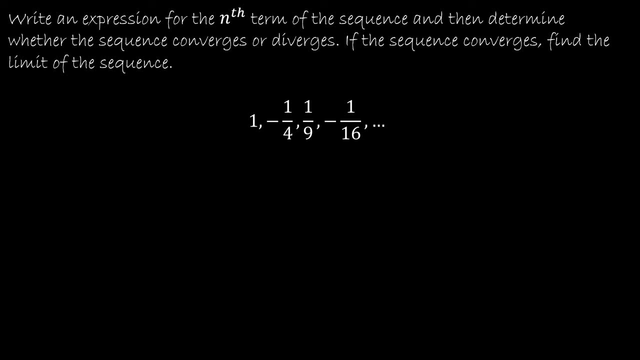 In this short video we're going to take a look at what happens when we're asked to find the limit of a sequence but we are not explicitly given the function that describes the sequence. For instance, in this example we are asked to write an expression for the nth term of the sequence. 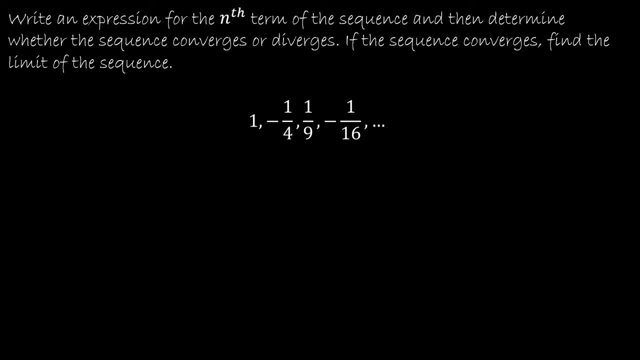 and then determine whether the sequence converges or diverges. So the problem here is that we are only given four values and we don't have some function or some expression that tells us how to find the nth term of the sequence. so that is what we'll have to do first, and then we can. 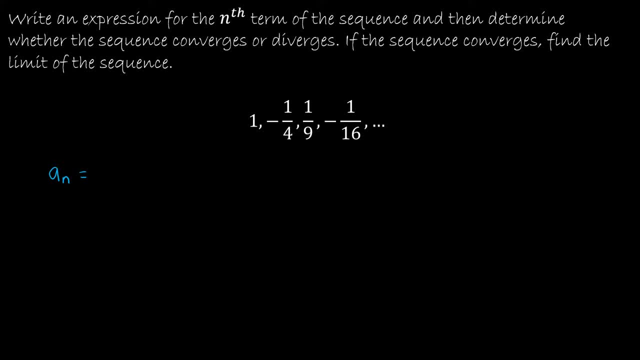 do all of the things we've just learned how to do, which is then find the limit and determine if it converges or diverges. So keep in mind that this guy would be a sub 1 and a sub 2, and a sub 3 and a sub 4, and there's different strategies for. finding t terms of the sequence. so just to give you a little general idea. else, funcありがとうございました. I'm not going to extend any more words in the next Q&A recording And I will look at the questions I have for this tutorial later. so keep in mind that there is not a lot of information. 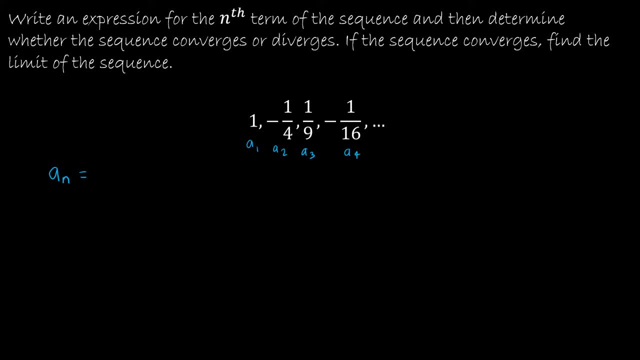 the pattern, but I can see, first of all, that this first term is positive and then negative, and then positive and then negative, and so one of the things that I'm going to use is negative 1 to the nth, and this is actually going to be negative 1 to the n minus 1. so we're always going to use negative 1 to some. 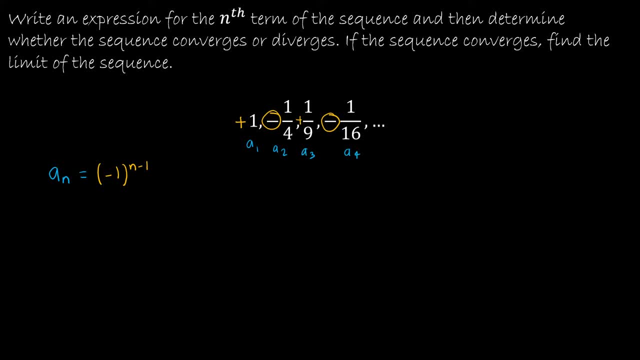 power if the sequence alternates like this. but you have to keep in mind whether or not this first value is positive or negative. so, since my first value is positive, if I would have had negative 1 to the n, then negative 1 to the first would give me negative 1 and I need it to be positive. so I'm just going to use 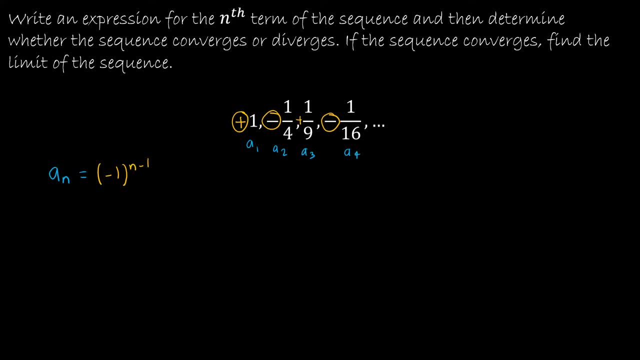 negative: 1 to the n minus 1 from here. now I need to take a look at the other part, so the other part is disregarding the positives and negatives. I have 1, 1 fourth, 1 9th, 1 16th, and this looks like 1 over 2 squared and this looks like 1 over 3. 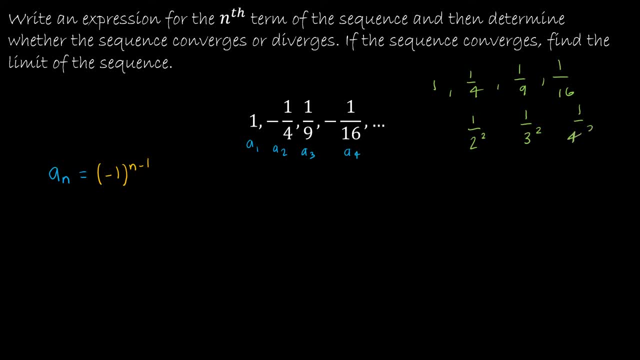 squared and this looks like 1 over 4 squared and I could write this as 1 over 1 squared. and so now I have to think about how could I write that in terms of n, where, of course, n here is 1 and n here is 2 and n here is 3 and n. 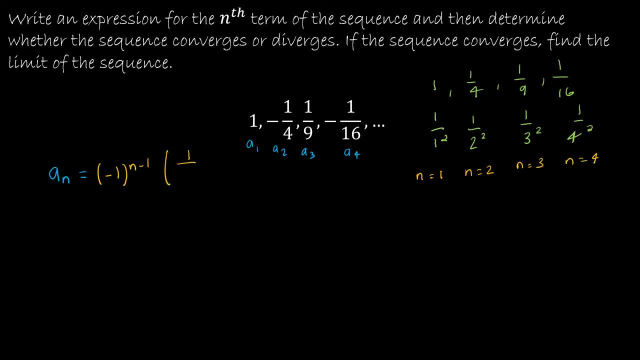 here is 4, so obviously this is going to be 1 over n squared. now it's always a good idea to then double check, especially when you're dealing with one of these guys, because it's very easy to forget and put the wrong n or n minus 1. 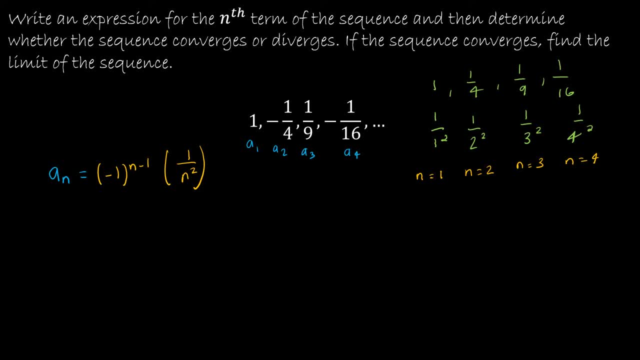 so it's not a bad idea to just double check. did I do this right? so let's just check a sub 3. negative 1 to the 3 minus 1, 1 over 3 squared. now I'm going to do a subtraction so I should end up with 1- 9th. so let's just make sure: negative 1 to 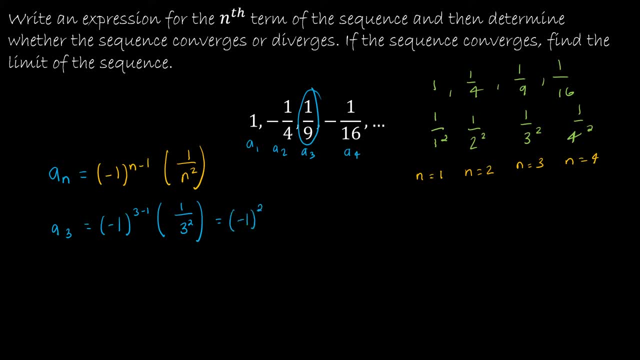 the 3 minus 1 is negative 1 squared and then 1 over 3 squared is 1- 9th. negative 1 squared is positive 1 and 1 times 1- 9th is 1- 9th. so I feel pretty good and 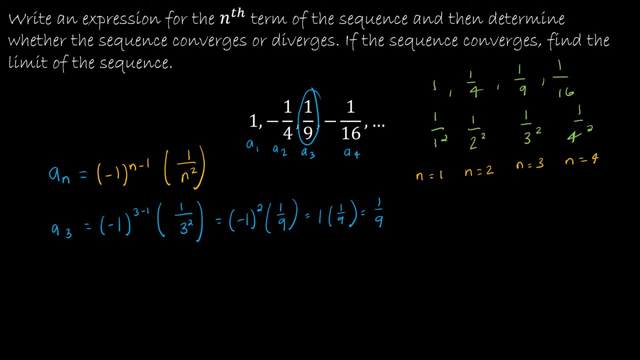 again. I could check as many as I needed to, but I'm going to stop there. so I've done the first part, which said: write an expression for the nth term of the sequence. the second part says: and then determine whether the sequence converges or diverges. so now that I have this, 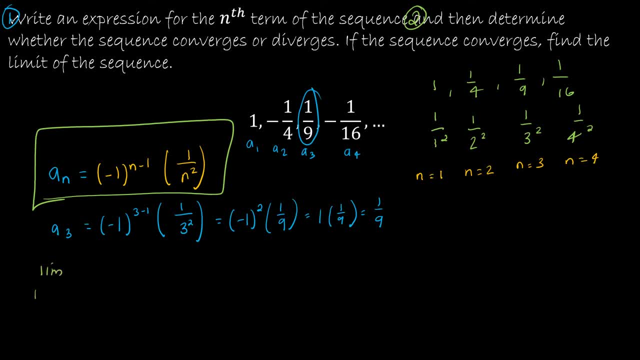 expression. I'm going to find the limit, as n approaches infinity, of negative 1 to the n minus 1, 1 over n squared. so finding the limit of this. again, I'm going to be thinking about the expression for the nth term of the sequence and I'm going to 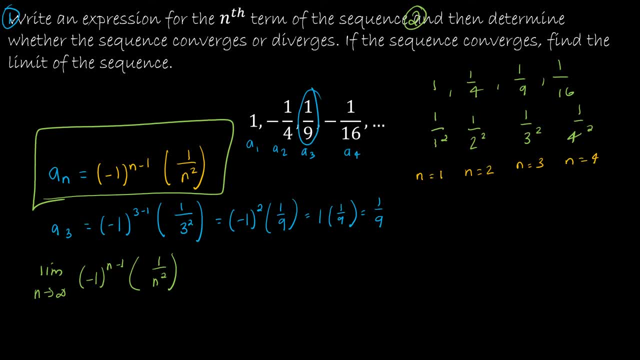 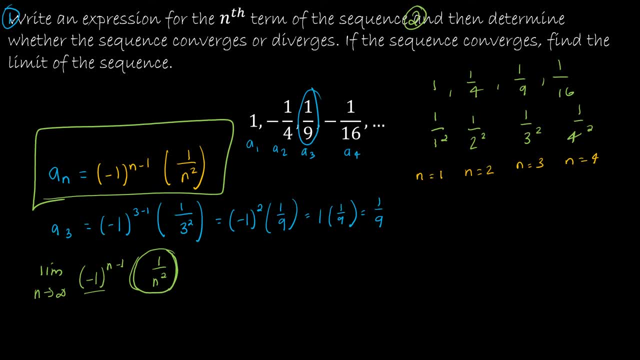 keep going back and forth from negative to positive. don't let that throw you off. This guy is certainly approaching zero, because this is essentially 1 over infinity And as that denominator gets larger, I am dividing by a larger number and getting zero. So this limit is in fact. 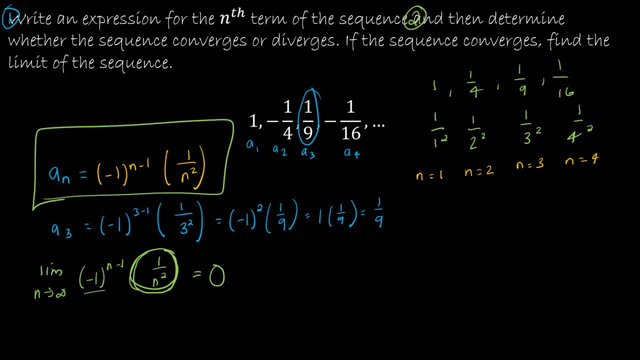 zero. Now again, I want to go back before we talk about converges and diverges, because obviously this converges, Remember it. converges if we have have a limit and we do have a limit of zero. But I do want to talk about this guy because a lot of 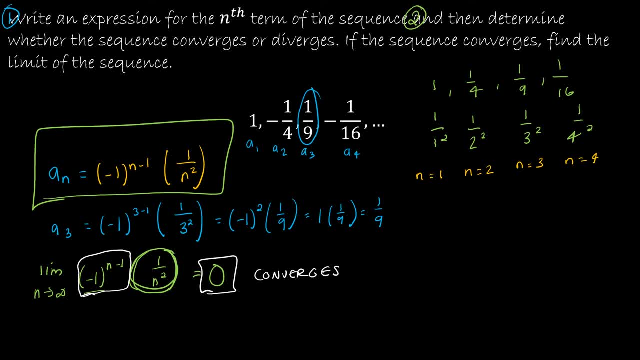 people get thrown off by that and say: well, how can it converge if it's going back and forth between positive and negative values? So if I think about graphing something like this: at 1, the value was 1, and at 2, the value was negative 1. fourth, and at 3, the value was positive 1 ninth. 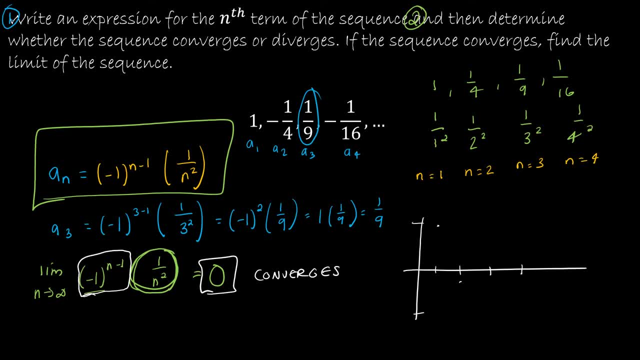 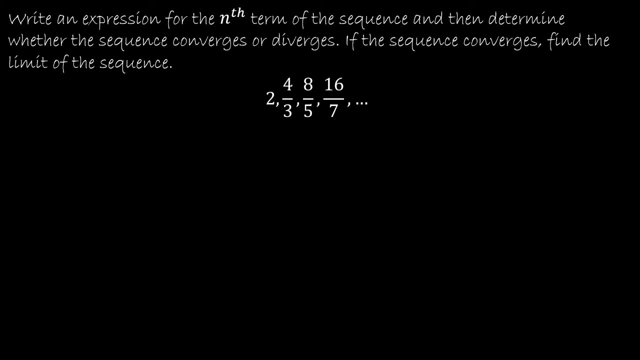 and at 4, the value was negative 1 sixteenth, And so I can see that, basically, what's going to happen is it's going to just start getting very, very small, and that's why it makes sense that this converges to zero. Here's another example. This one is a little bit tougher, just because you're. 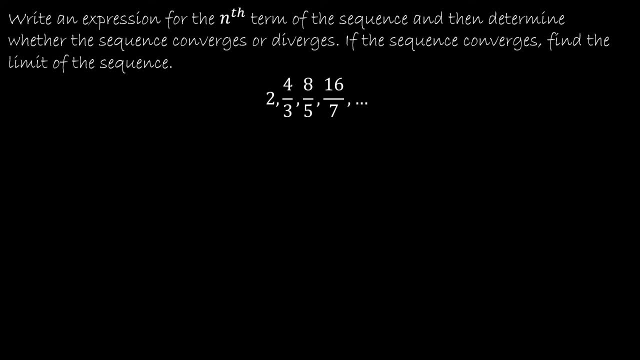 going to have to think back to some things you learned in Calculus 1, which is, of course, why I included it in this video, so that I could refresh your memory. So if you're feeling up to a challenge, press pause And try this one on your own, And if you're not feeling up to a challenge, then let's just get started. 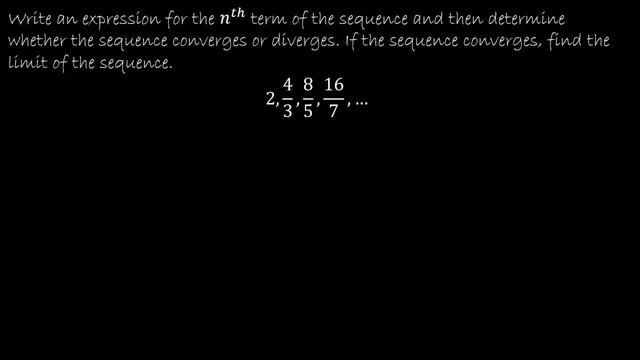 together. So, to begin first, we're going to write an expression for the nth term of the sequence, That is step 1.. So, again, I'm going to take a look at what kind of pattern can I find This? 2, I'm going 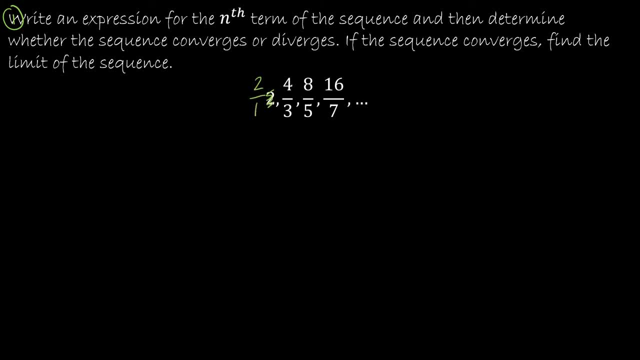 to write as 2 over 1, because obviously these are all fractions. So, as I'm thinking about a sub n, I'm going to have some expression in the numerator and some other expression in the denominator. So, focusing first at 2, 4,, 8,, 16, that appears to follow a pattern of 2 to the first, 2 to the second, 2 to the third. 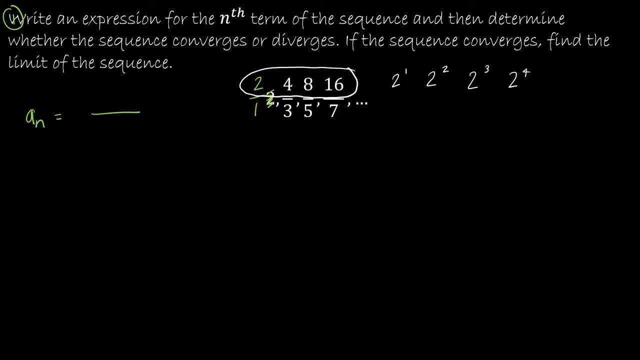 2 to the fourth, and since this guy is n equals 1, and this is n equals 2,, and this is n equals 3, and this is n equals 4,, it seems that I could write this as 2 over 1.. 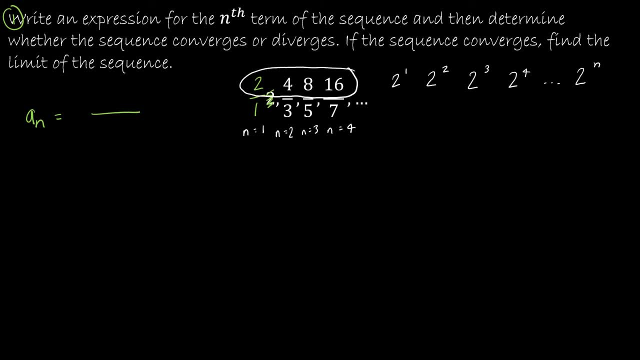 05. 06. 07. 08.. to the n. So that's my numerator In my denominator, again keeping in mind, I'm writing it using n. so looking at this pattern, obviously from 1 to 3 I increased by 2, from 3 to 5, I. 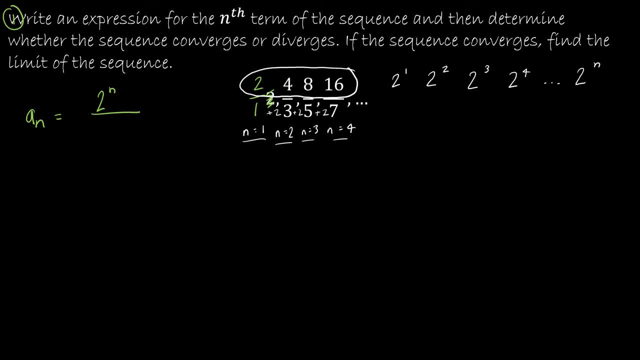 increased by 2, from 5 to 7 I increased by 2, so that tells me that I'm probably going to have 2 times n happening somewhere. Let me move that down. 2 times n Now if I plug in 1,. 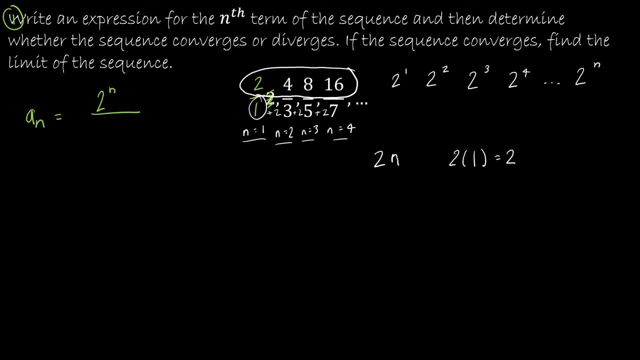 2 times 1 is 2, but I need it to be 1.. So how about 2 times n minus 1?? So that's 2 times 1 minus 1, would be 2 minus 1 or 1.. So that gives me my first value: 2n minus 1. 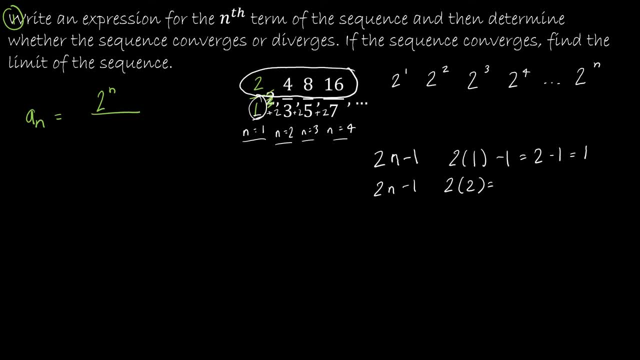 for 2 would be whoops, 2 times 2, which is 4, minus 1, which is 3.. And so I feel pretty good about it, that I have come up with the correct strategy and that tells me that this guy is 2n. 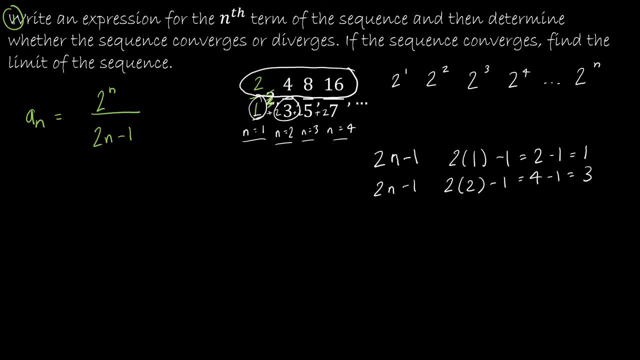 minus 1.. And again, you are welcome, before you get started on the second part of this question, to just choose a value at random, Let's say a sub 3, and see does that work. So 2 to the third times, or over 2 times 3 minus 1 would give me 8 over 6 minus 1, which is 5. 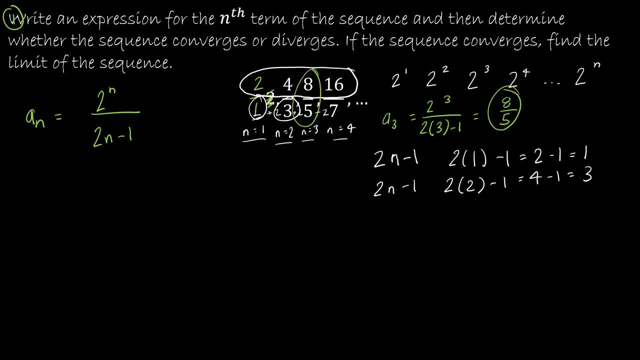 and 8 fifths is in fact the third term. So that's step one is. I've now written this sequence basically explicitly so that I could find each value using some function. Now I want to determine: does the sequence converge or diverge? And if it converges, what's the limit? So I'm going to find the limit as n approaches. 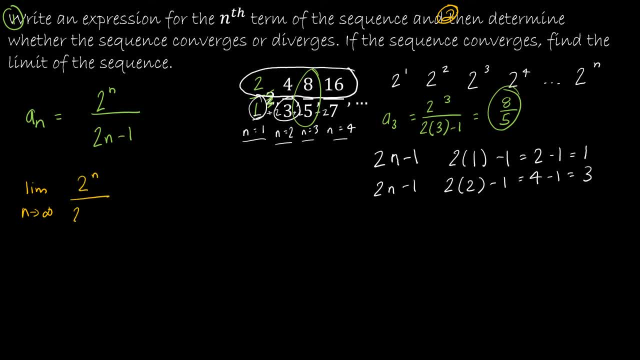 infinity of 2 to the n over 2n minus 1.. Again, direct substitution here would be a dumpster fire. You're just going to get 2 to the infinity and 2 times infinity. That's just a lot of infinities, And so I purposely threw this one in here, and this is why this one is more. 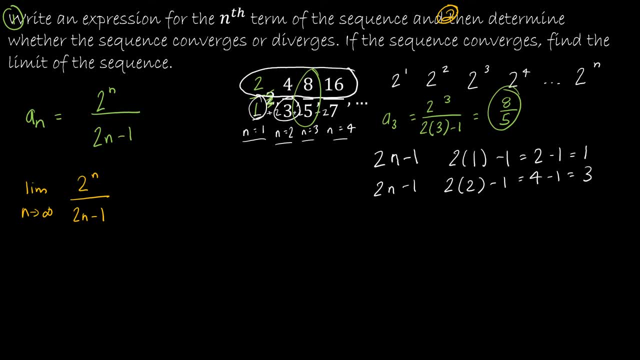 difficult is. I want us to think about some other strategies for finding limits When we can't find them by direct substitution. So we reviewed several in our last video, But in this video let's go ahead and take a look at 2 to the x over, 2x minus 1.. 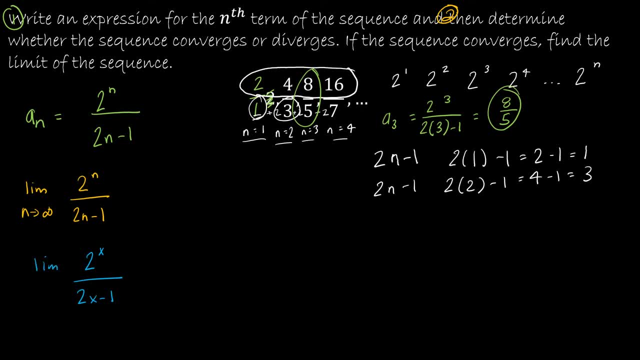 So, again, just using that rule that says the limit of the function is the same as the limit of the sequence. So I'm just going to think about this as a function. The limit, as x approaches infinity, of 2 to the x over 2x minus 1.. One of the strategies that we're going to use to 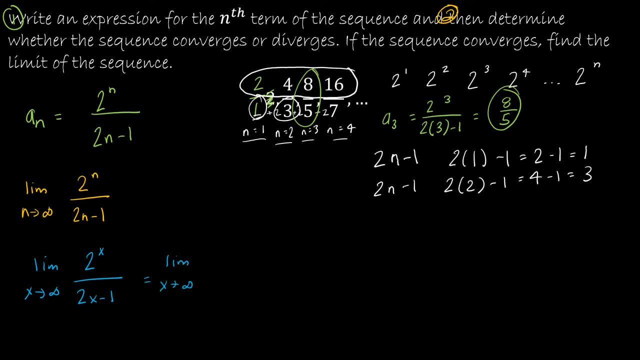 find the limit of the function is the derivative of the numerator and the derivative of the denominator. Well, what is the derivative of 2 to the x? The derivative of 2 to the x is 2 to the x times the natural log of 2.. So that's helpful, because now I'm only dealing with 2 to the x power. 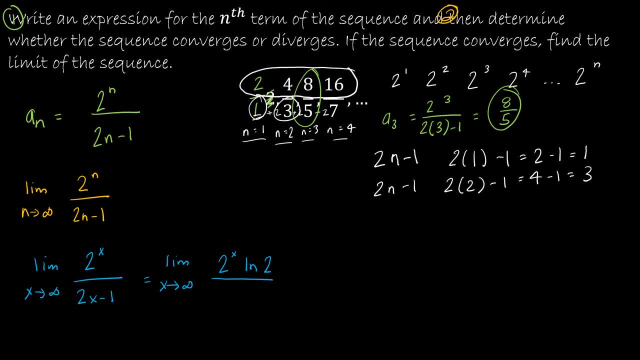 And in the denominator I've got 2x minus 1.. What's the derivative of 2x minus 1? It's just 2.. So that's super helpful, because now I no longer have a 2x in my denominator. I don't have an x in. 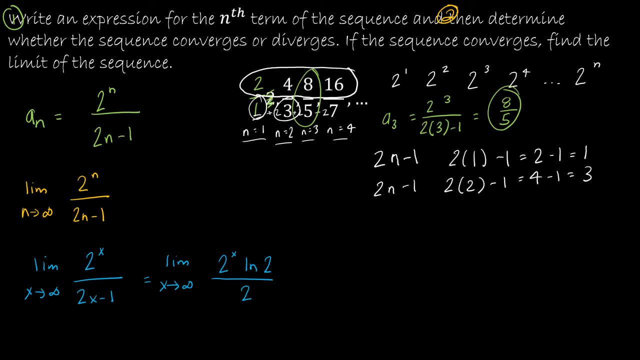 my denominator. So now what I'm doing is thinking about what's the limit of this function. Well, thinking about 2 to the infinity power, that means this guy in the numerator is approaching infinity. Natural log of 2 really doesn't affect us at all because I'm taking infinity times, some value. 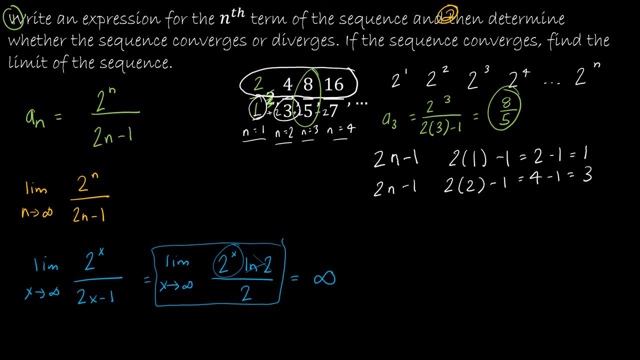 And then I'm dividing it by 2. I'm still going to approach infinity. So because that function approaches infinity, then the limit of this sequence is also infinity, which means this guy diverges. So again, what rule did I use? This was L'Hopital's rule that says you can take.